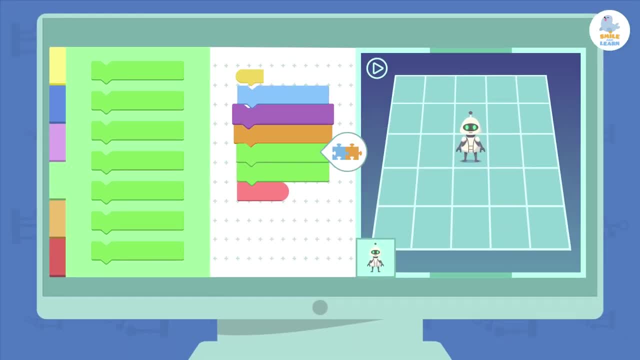 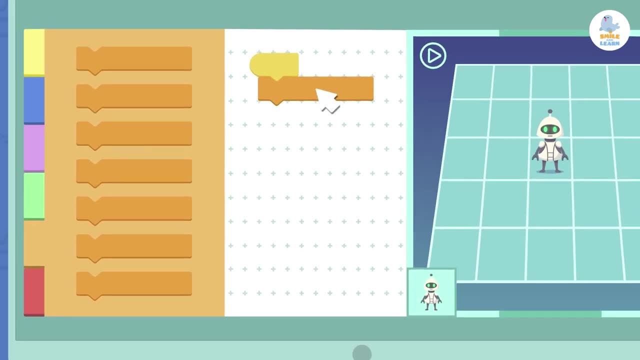 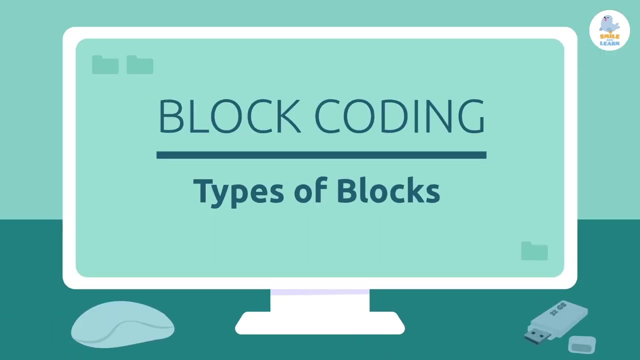 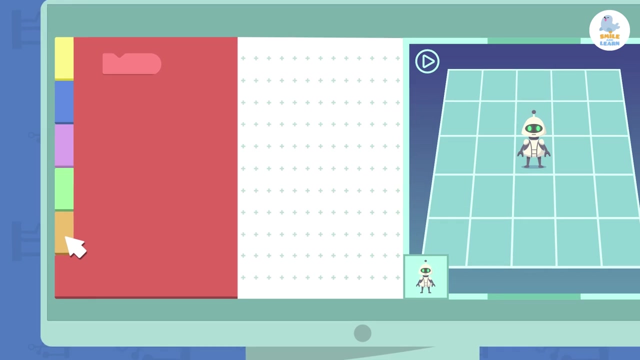 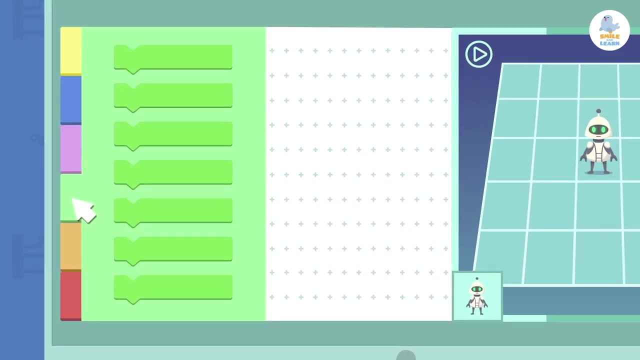 to organize the instructions you're programming. You can combine different blocks. Here you will find all the necessary components that you can select to make fun projects. There are different types of blocks and there are many different actions that you can choose from. On top of that, each block category has a different color to help you find them. 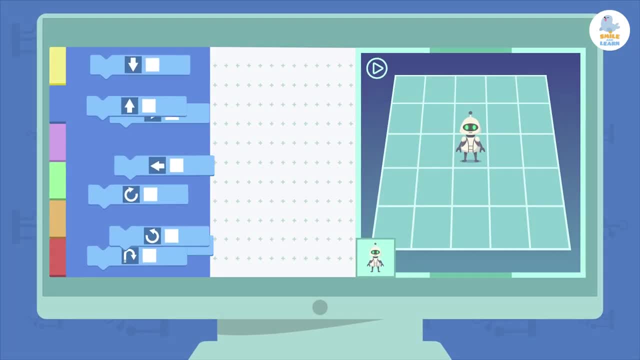 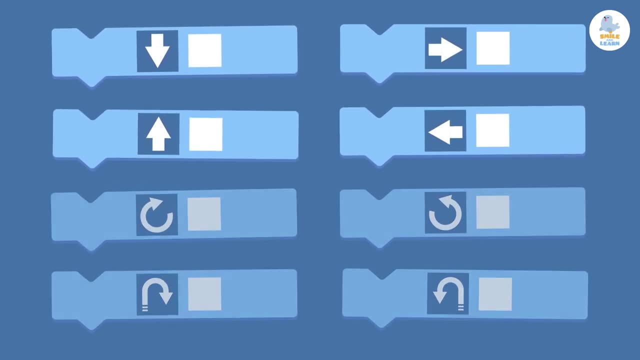 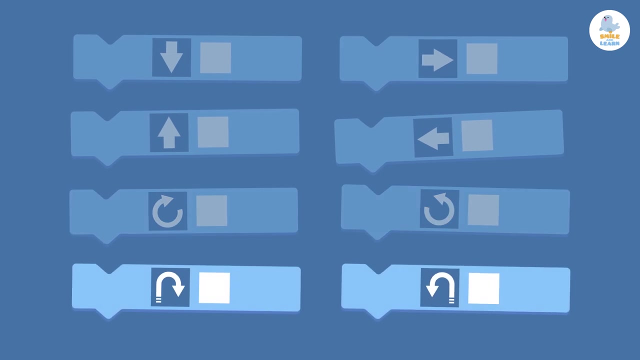 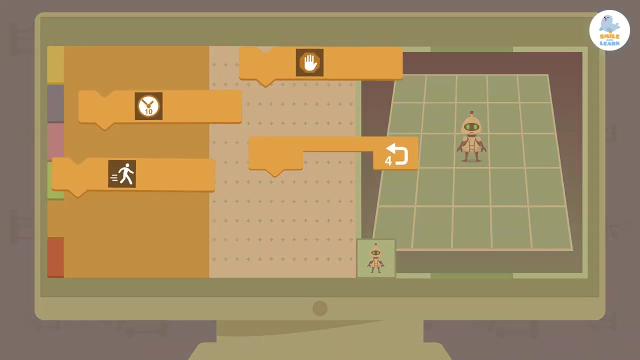 better. For example, Motion blocks are blue. These allow you to move a player or a robot from one place to another, As well as doing other movements such as turning, jumping or tilting. But there are also control blocks, which are orange. They help you repeat an action as many times as you want, and 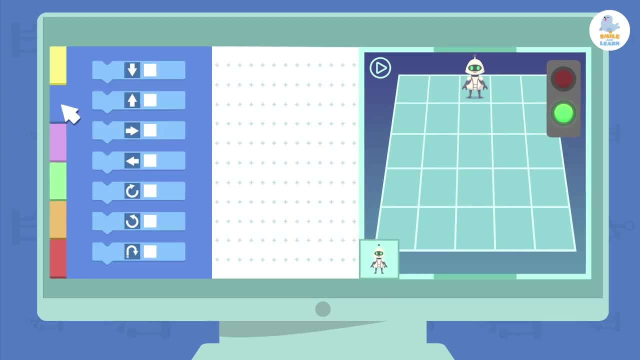 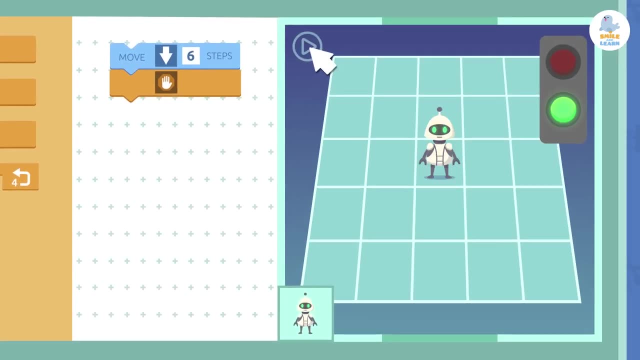 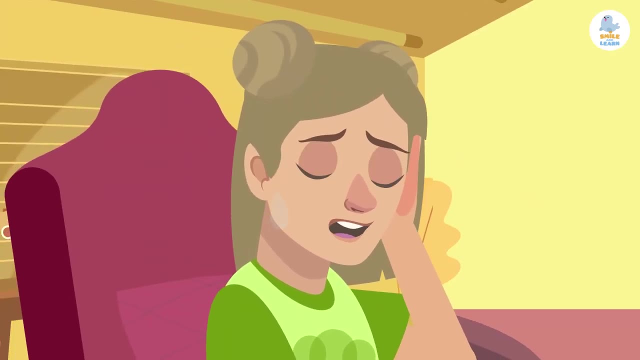 set conditions. For example, You can teach your robot to walk forward only when it sees a green light and to stand still if it sees a red light, just like a traffic light. So far at school, I've only been taught how to program using the most common movement blocks. 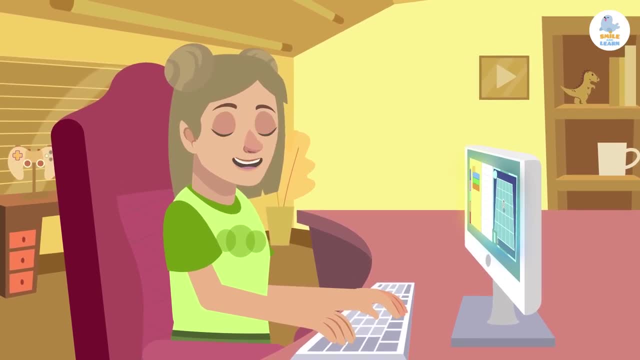 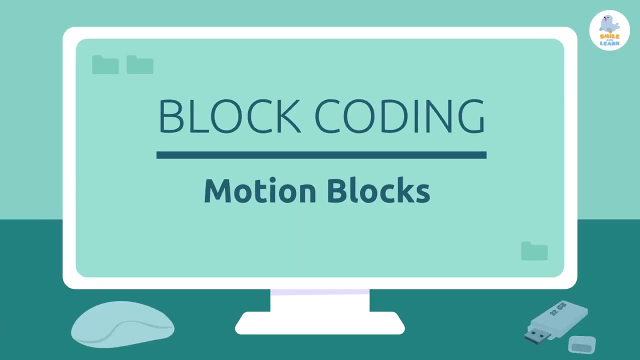 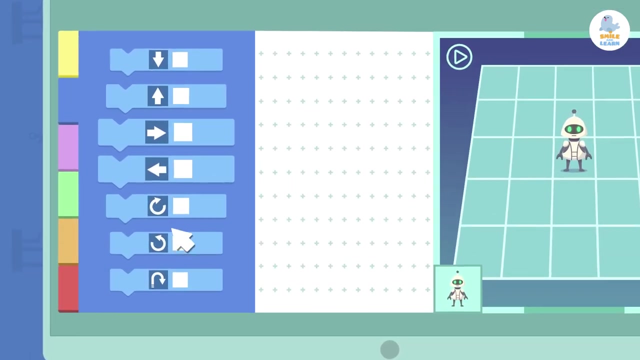 These blocks allow me to tell my player how I want it to move. So do you want to see how I teach my player to dance, To move it? you could use different motion blocks. The most basic ones are those that allow you to move. 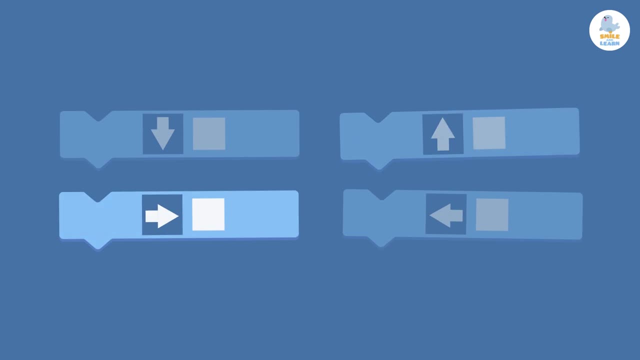 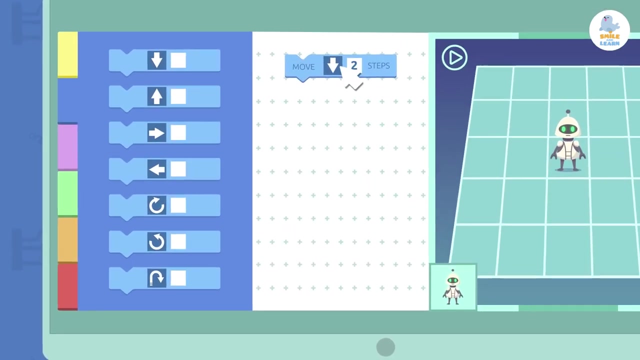 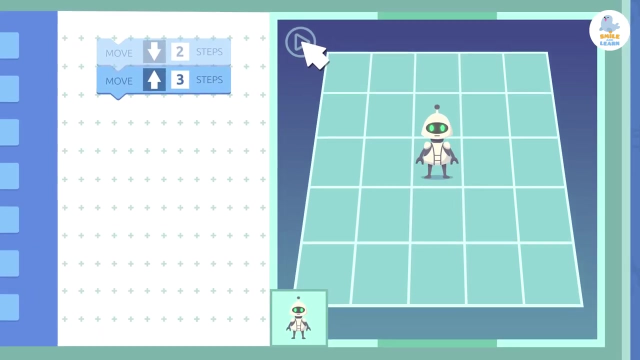 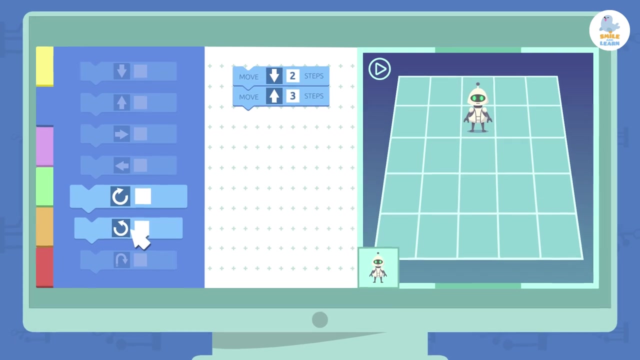 Forward, backwards, to the right and to the left. First I'll program my player to take two steps forward and three steps back. Look closely: As well as motion blocks, we can also find rotation blocks. Can you think of why? 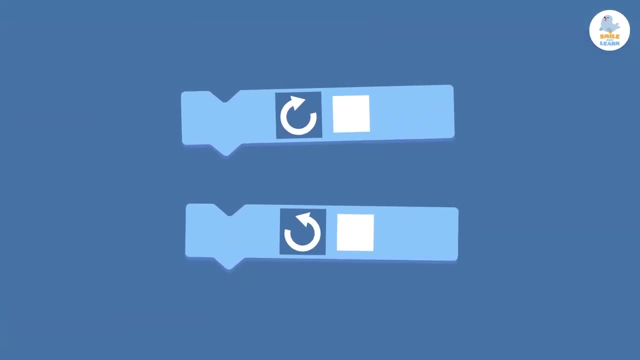 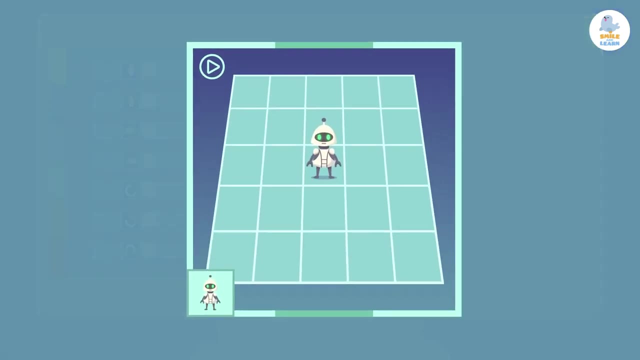 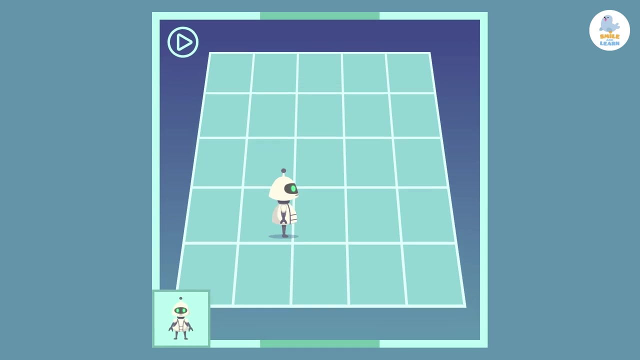 Normally there are two types of turning blocks used: Turning to the right and to the left. The turning blocks help us have a more natural movement. They allow us to rotate our player's body, to change the direction of its movement. We'll program the player to take two steps forward.